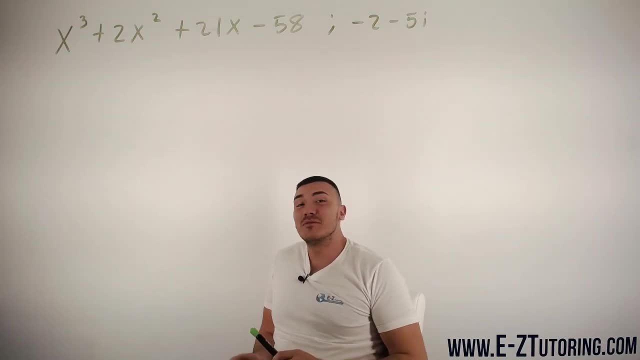 Hi and welcome to EZTutoring. Today we are going to figure out how you can find your remaining zeros when you are given one complex zero, And this is the complex zero that we're given. So here's a good rule of thumb Whenever you're given a complex root or a complex zero. 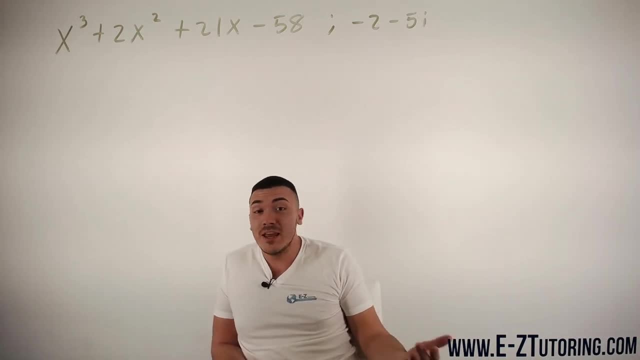 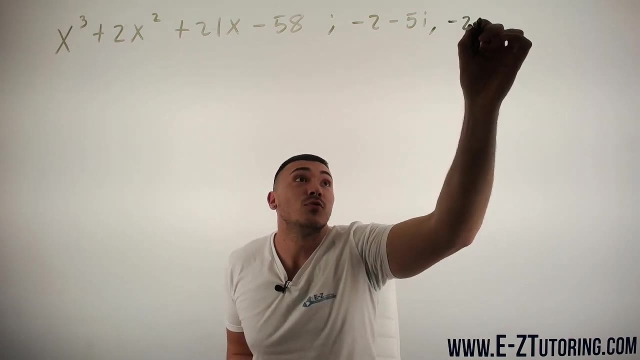 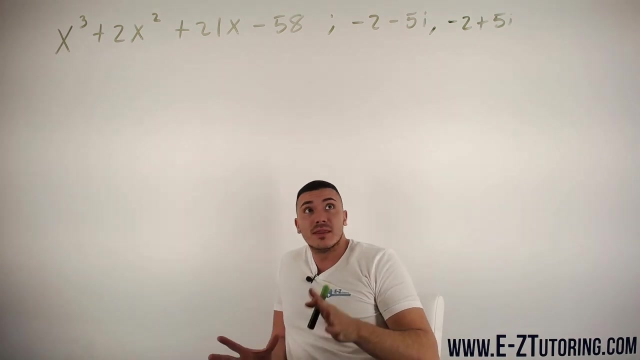 its conjugate will always be a root as well. So if we're given negative two minus five, we can automatically assume that negative two plus five i will also be a zero, And that is for every polynomial. this rule always applies, and this should be automatic Every time you see your. 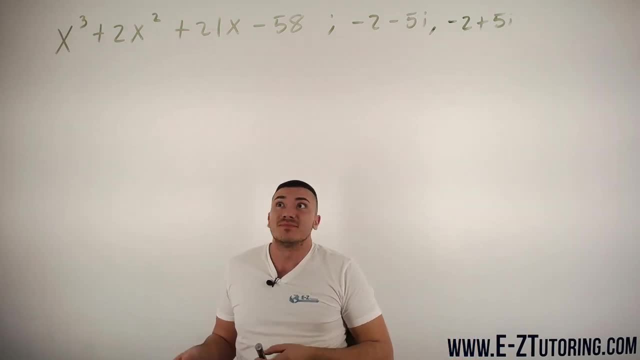 complex root, always take the conjugate and say that that's a root as well. Alright, so are we done? Well, this is x cubed, which means we have three roots, and so far we have two. we have one left, So normally, 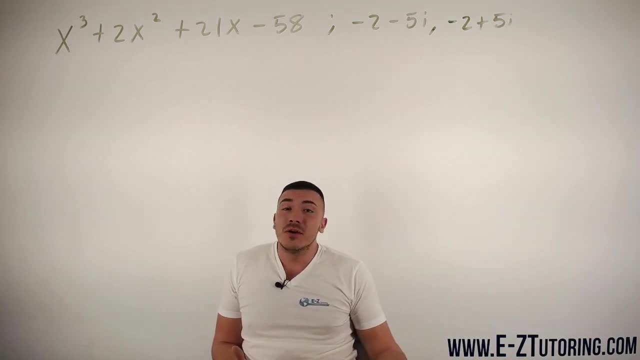 if you see my video on how to find the remaining zeros, you know that you would use synthetic division, divide by your root and see what you're left with. But in this case, can we use synthetic division with a complex number? Yes, you can. Is it recommended? No, it is not. You can do it. 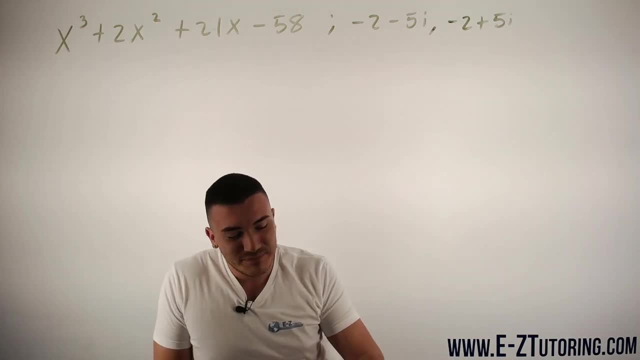 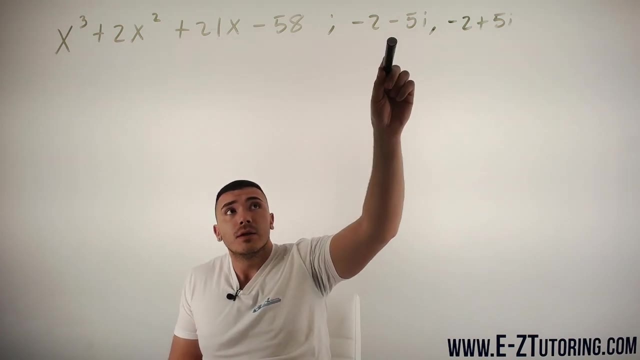 you will find your answer, but I will show you guys a better method. So the better method. what you want to do is you first want to realize that your root. if you put it in a binomial, it would just be x minus. whatever your root is. 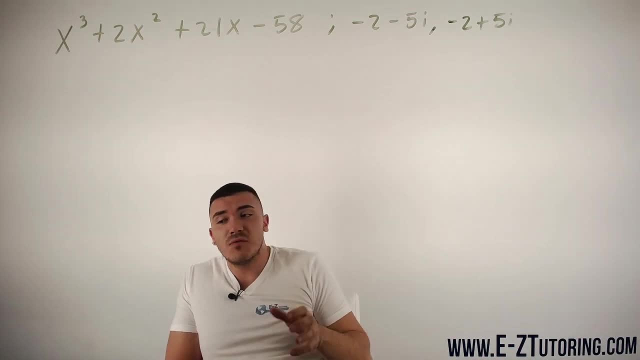 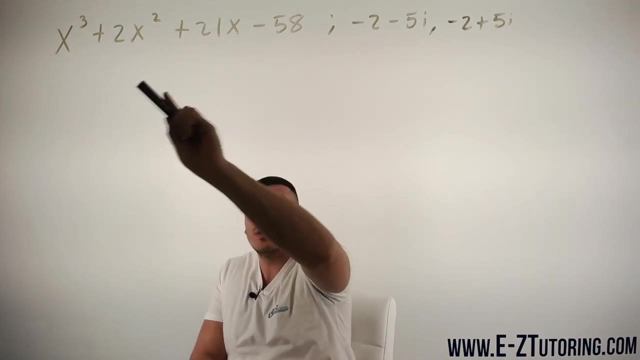 In this case it would be x minus all of this, And if we take x minus of every root and we multiply all of our three roots together, we would get this entire polynomial. Now we don't know what our third root is, so let's just go ahead and multiply. 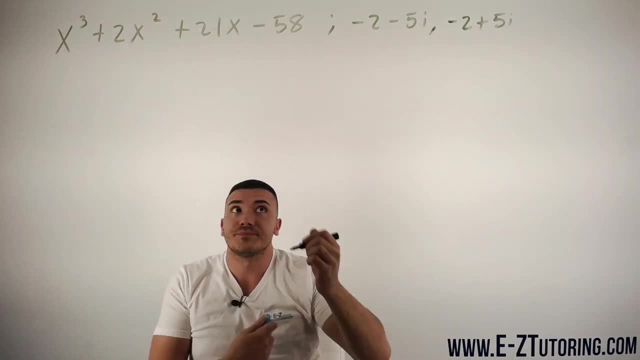 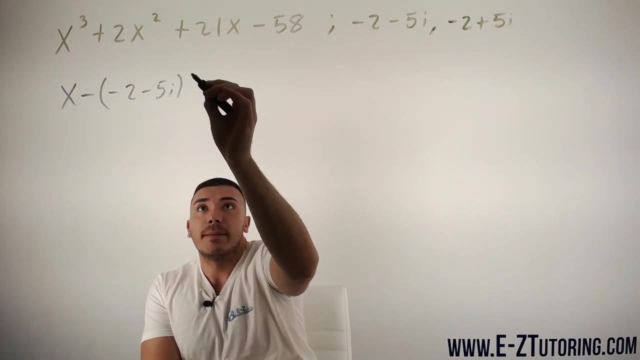 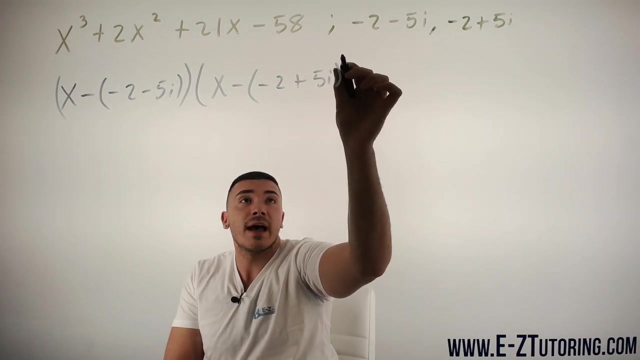 these two first and we will be close to that polynomial. So we will have: we have x minus this root negative two minus five i, And x minus this root negative two plus five i. So we're gonna go ahead and multiply these two together. 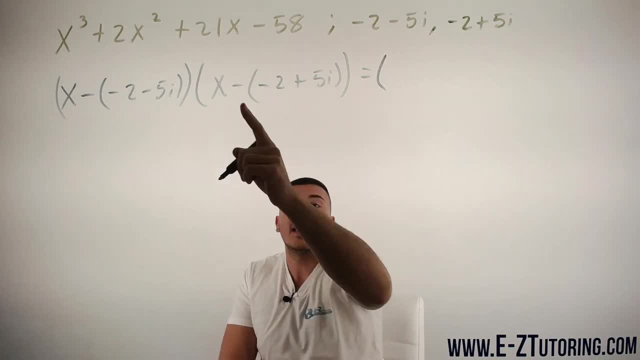 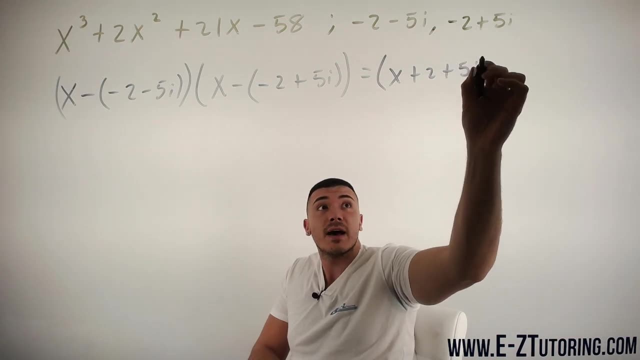 Now, what I'm going to do first is I'm first going to distribute these negatives in there, just to make things not so complicated. First one gives us x plus two plus five i, And the next one gives us x plus two minus five i. 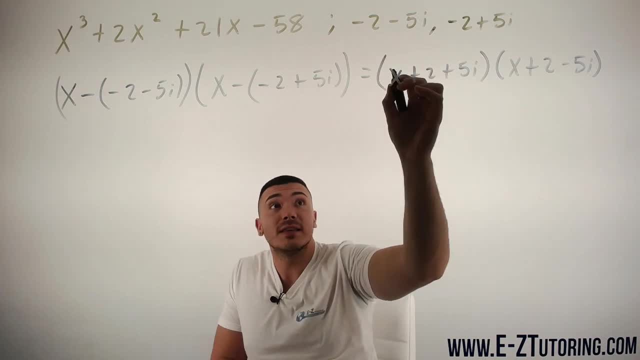 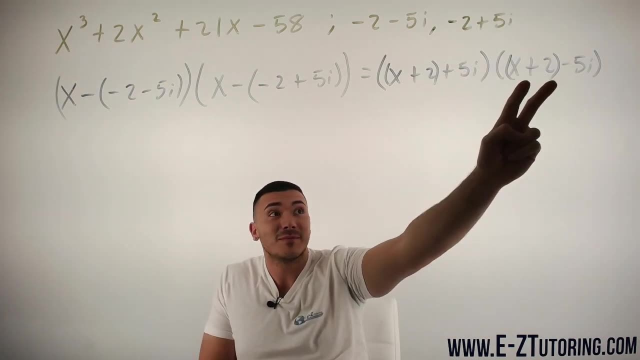 So now what I'm going to do is I'm going to put parentheses around the first two terms: x plus two. Why did I do that? X plus two and x plus two are the same. Five i and negative five, i have the difference. 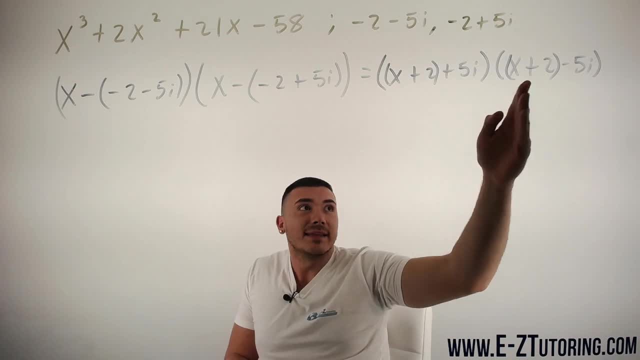 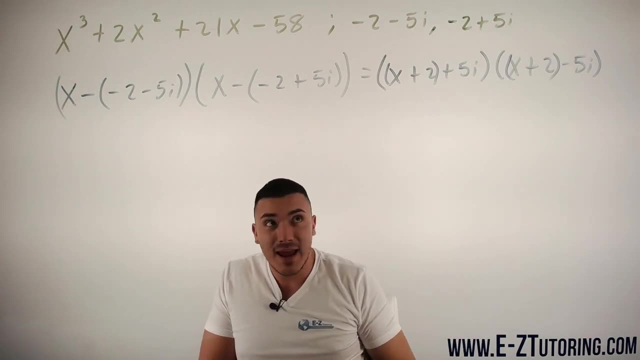 of a negative. This is like saying x plus a, x minus a, and whenever that is the case, you will get the difference of squares. You end up foiling it out. You'll see what I mean in a second. I just want to explain why I'm doing what I'm doing. 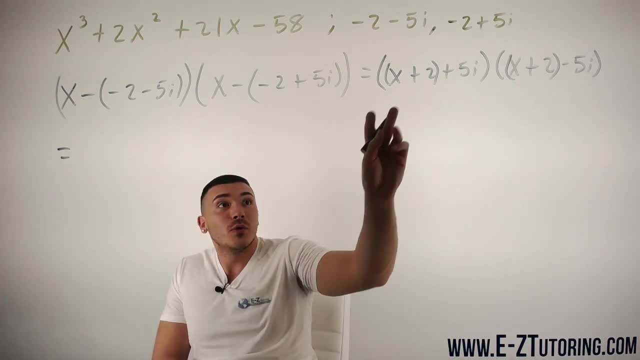 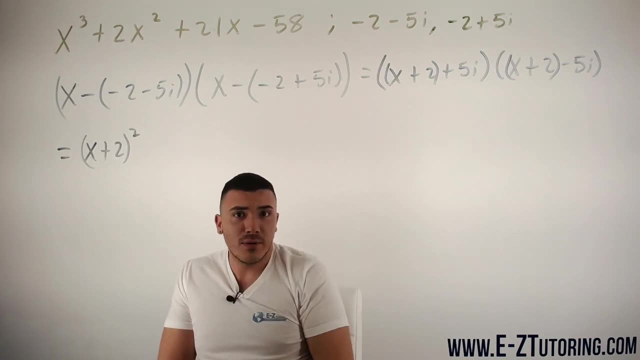 So when we go ahead and foil this out, we will do x plus two times x plus two, which is x plus two squared. We'll figure out what that is a little bit later. Then this is what I was talking about. 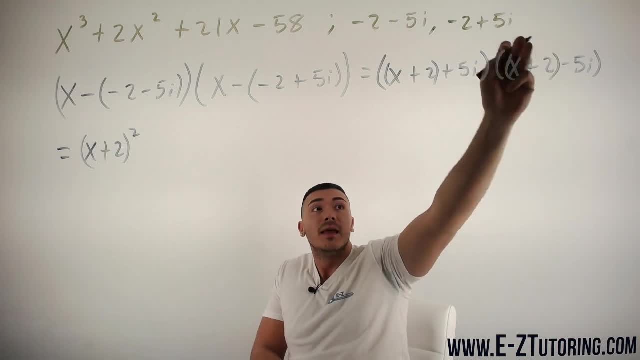 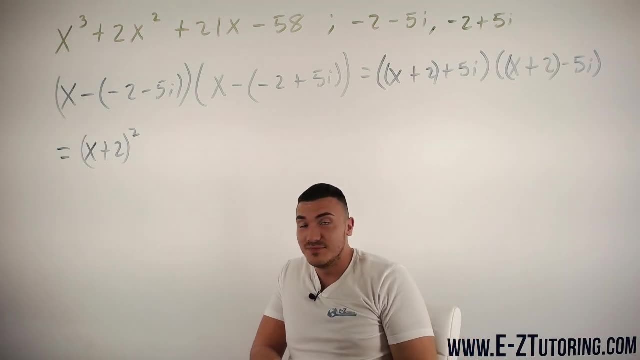 X plus two times negative five. i plus x plus two times positive five. i. Those two terms will cancel. I'm not going to write it out just to save some time. but if you guys don't believe me, which I recommend that you do believe me- 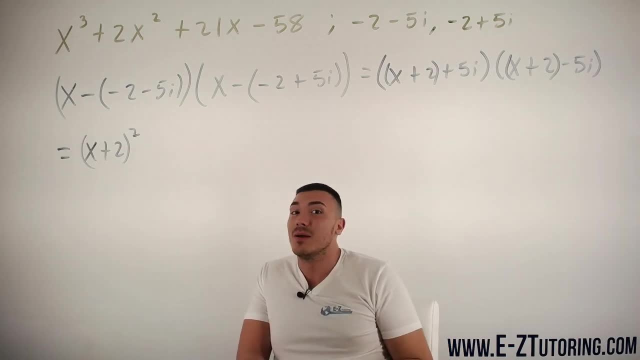 you can actually go ahead and foil this out and see how the middle two terms will cancel out. So then, all we got to do is multiply the five i and negative five i, which gives us negative 25. i squared- i squared is negative one. 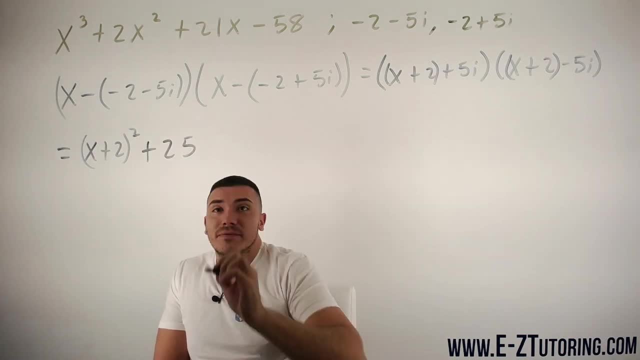 Negative one times negative. 25 is positive 25.. I don't want to focus on the x squared. I want to focus on the x squared. I don't want to focus on the little stuff here, like the little i squares and stuff. 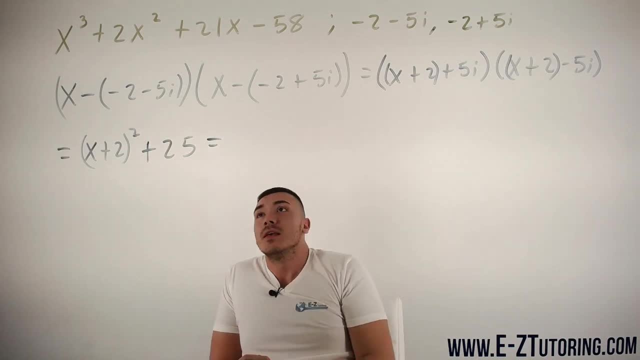 I mainly want to focus on the algebraic stuff. So, from here, what I'm going to do is I'm going to write out what x plus two squared is. It's x squared plus four, x, and then it would be plus four. 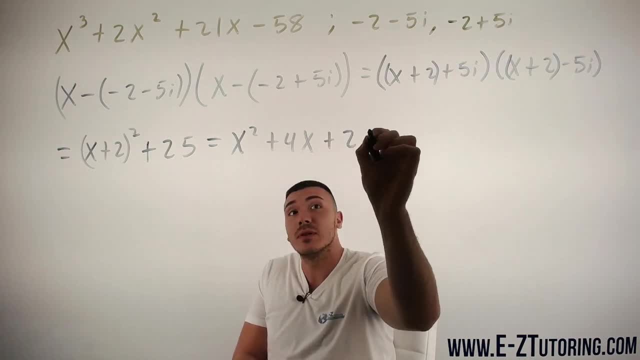 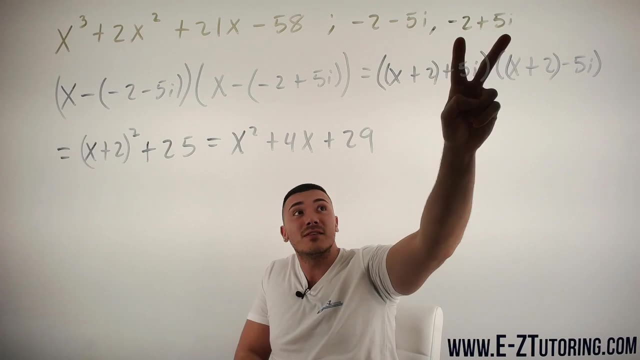 But I'm going to go ahead and combine that plus four with the plus 25, which gives us plus 29.. All right, so now we know that when you multiply this root in binomial forms, you will get x squared plus four, x plus 29.. 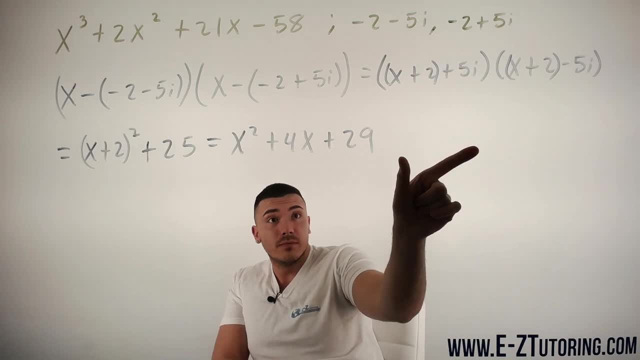 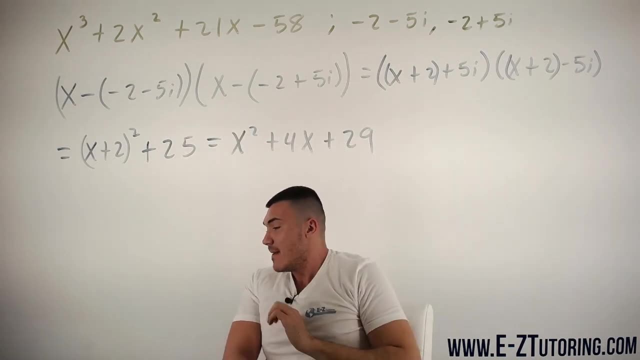 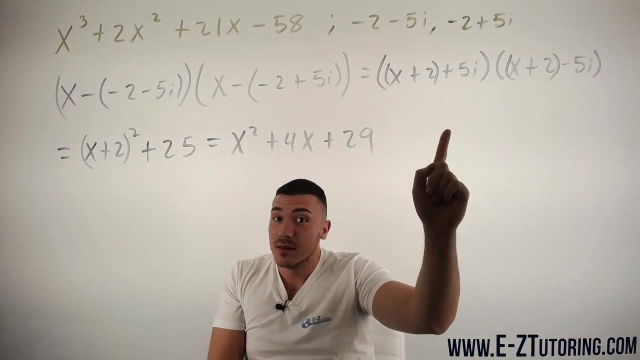 So if we were to multiply our last root, x minus whatever the last root is, we would definitely get the original polynomial we started with. No doubt about that. This concept is very important to understand for what we're doing here This times. something equals this: 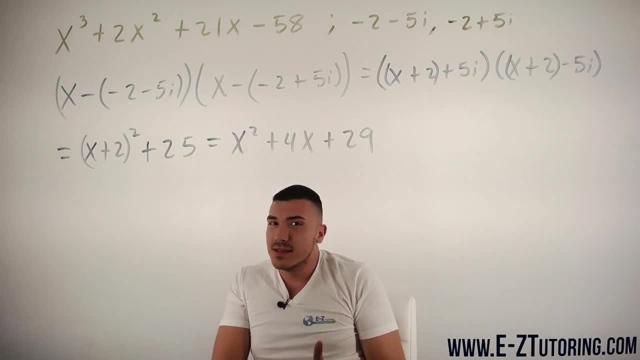 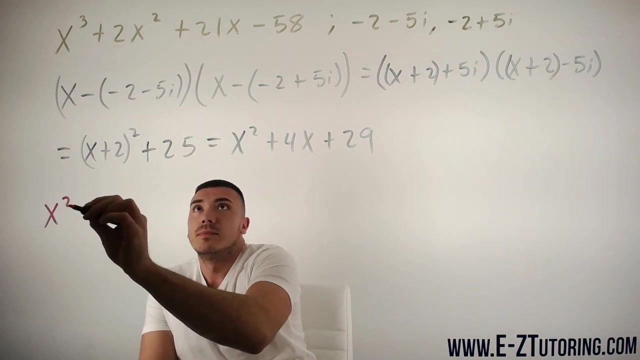 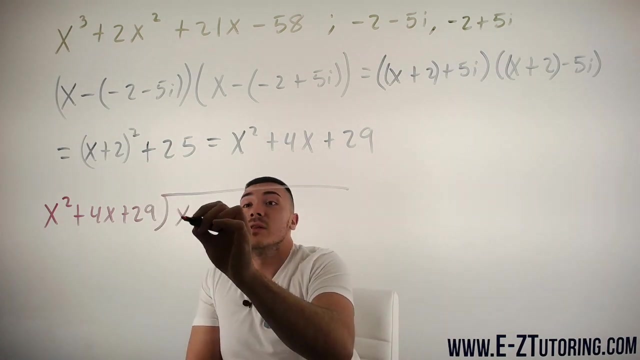 So now that you understand that, then that means that this divided by this will be equal to the last root, That one last root that we need to multiply by. So, like I said, the original polynomial divided by this will give us that last root that we are looking for. 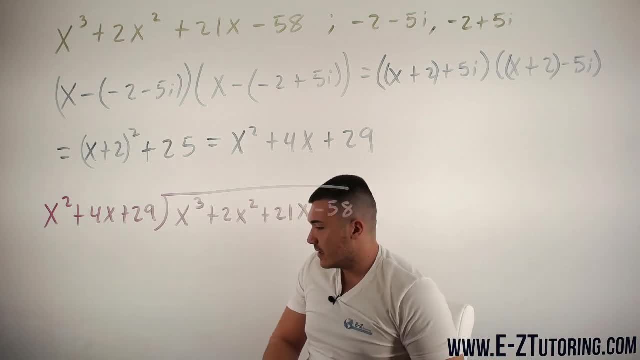 So, before you move on, before you continue this video, I really recommend understanding this concept that I just explained. If you understand this concept, great, and it's time to move on. Time to divide this into here. I'm not going to explain how to do polynomial division. 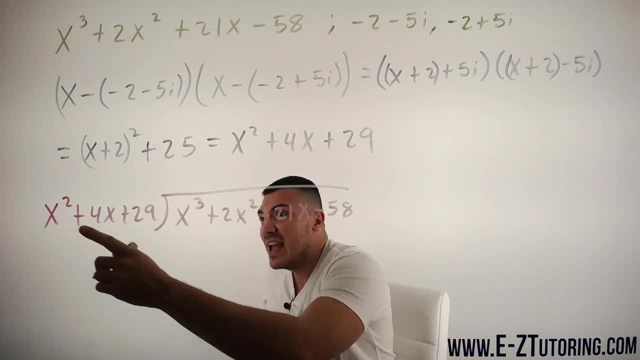 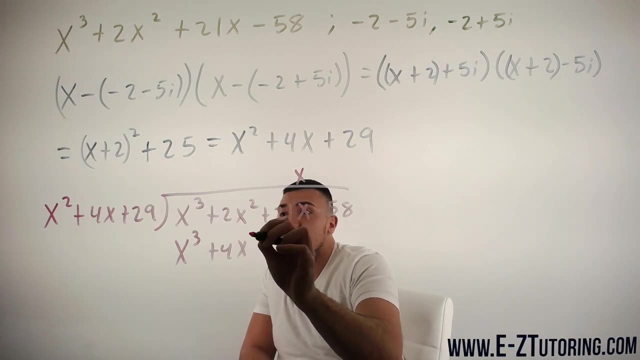 If you guys don't know, be sure to check out my video on it. So x squared into x cubed goes in x times x times. all that is x cubed plus four, x squared plus 29x. Subtract all of this. 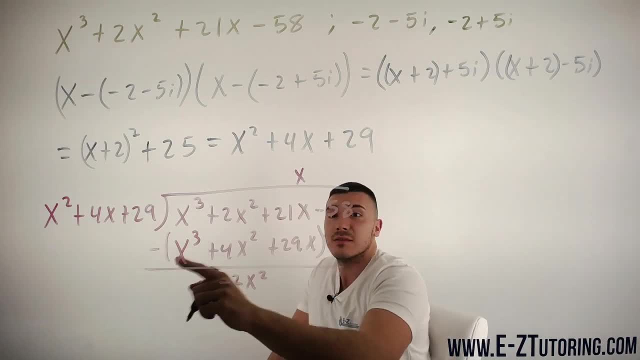 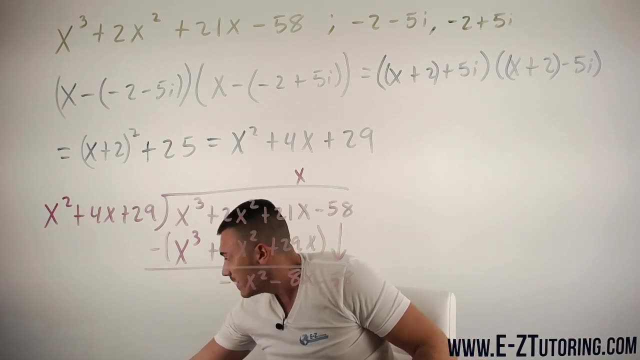 Two x minus four x squared is negative two x squared This minus that is negative eight x. Bring down the negative 58 at supersonic speed And then we have to see how many times does this go into here. Goes in negative two times. 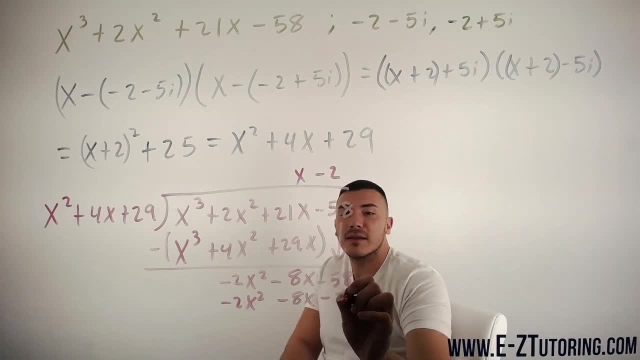 Then we'll get negative two x squared minus eight x minus 58.. Subtract all of this to get a remainder of zero, which means it worked out perfectly And we're done. And that means that this is our last factor. This is the last root that we were looking for. 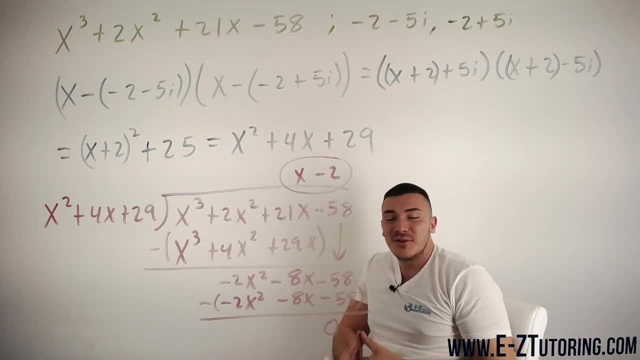 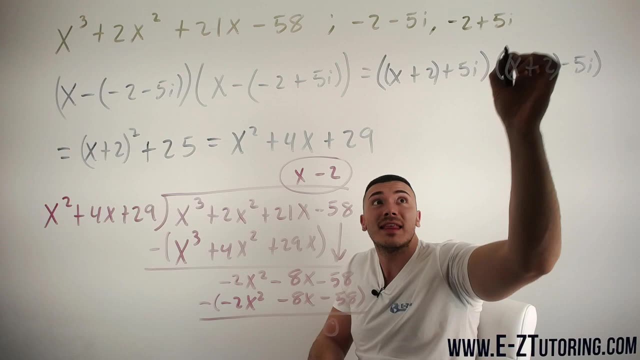 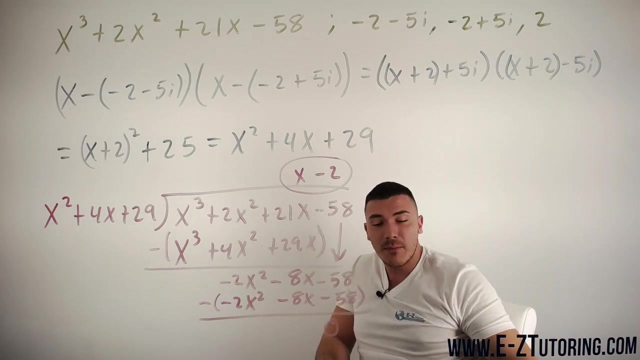 So from here you can find your remaining root. All you do is take x minus two and set it equal to zero. And when you set it equal to zero, you will get that x equals two. So from here, just to sum up everything: